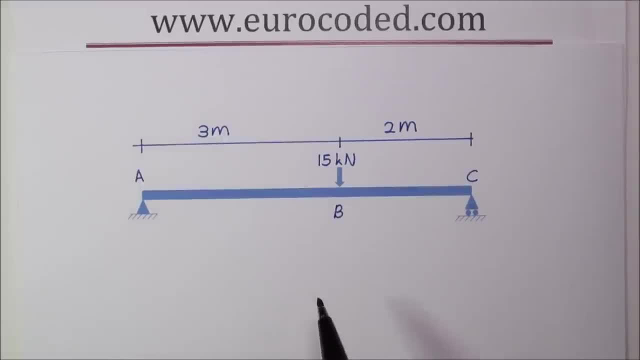 In this example, we are looking at a simply supported beam. As you can see, it is a five meter long beam and we have 15 kilo newton load applied at B. Distance from A to B is three meters and from B to C is two meters. It is simply supported with a roller support at this end. 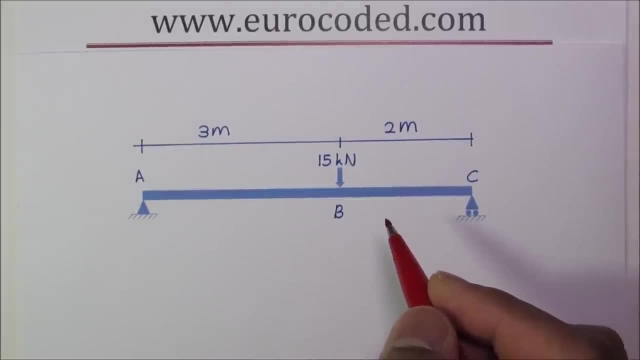 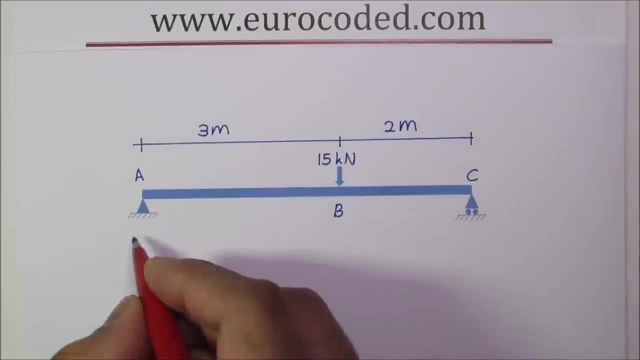 We only have one vertical load applied onto the beam at B, Hence we would only have vertical reactions at A and C. If I note them as R A and R C, then we can begin our calculations to determine the reactions at supports. What I'm going to do is take moments about A. You can see that the lever 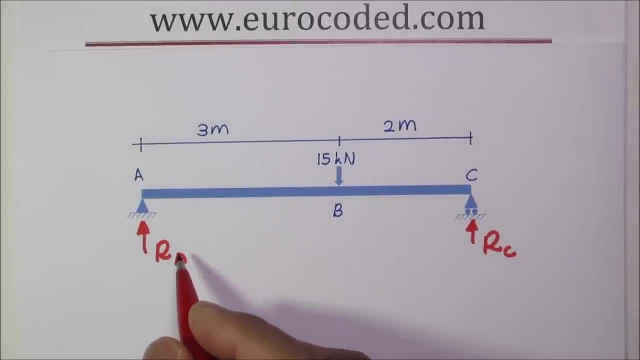 arm is zero for reaction B and C. The reaction to the beam is equal to zero for the support beam, RA, when you are taking moments about A, Hence RA has zero moment about A. We have an anticlockwise moment due to RC reaction and the lever arm is 5 meters. It's from A to C So we can write. 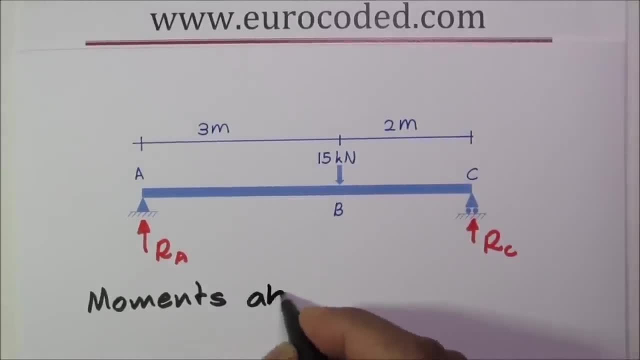 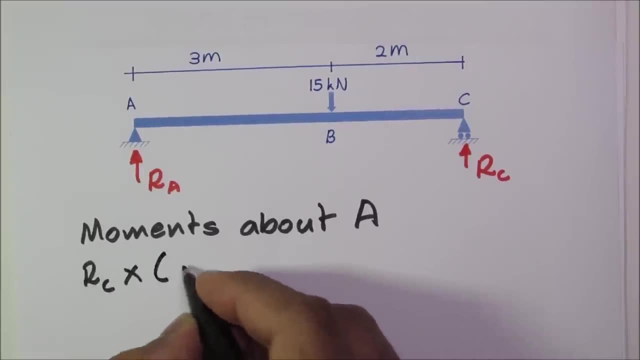 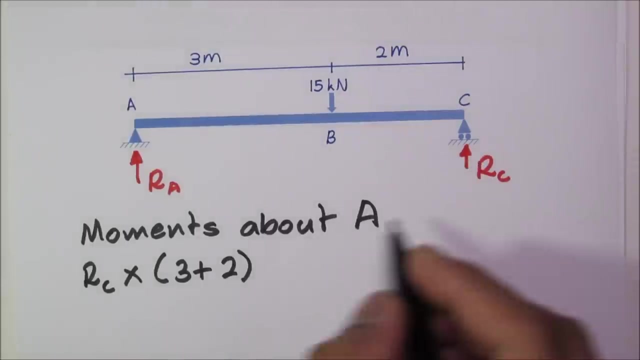 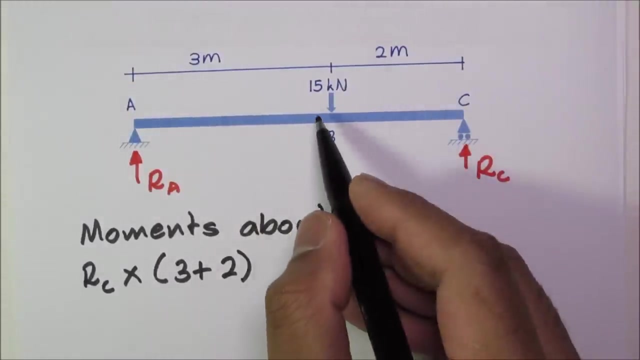 moments about A RC times 3 plus 2.. RC is causing an anticlockwise moment. As you can see, it would try to rotate this beam in this direction, anticlockwise. And then we have this 15 kilonewton force acting at B which is causing an anticlockwise moment. So we have an anticlockwise. 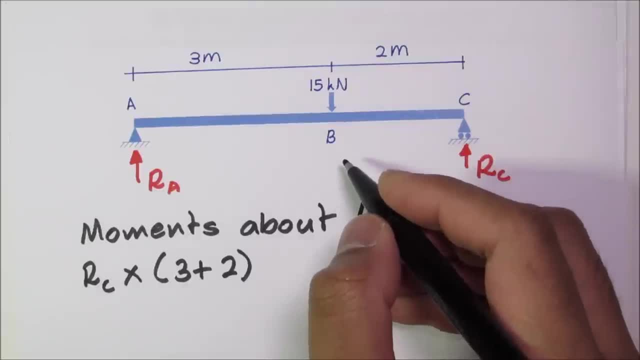 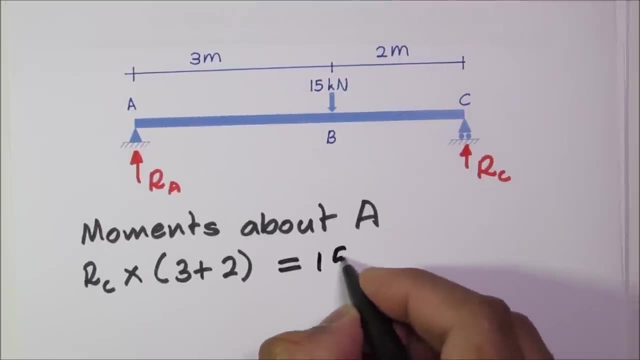 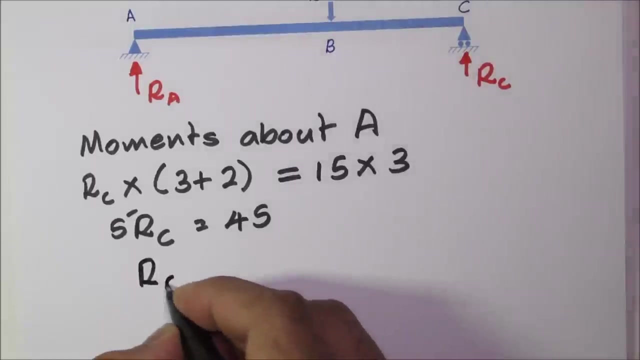 moment It would try to rotate this beam about A in this direction. So we can write: this is equal to 15 times the lever arm, 3 meters. You can write 5, RC is equal to 45 and RC is equal to 9 kilonewton. 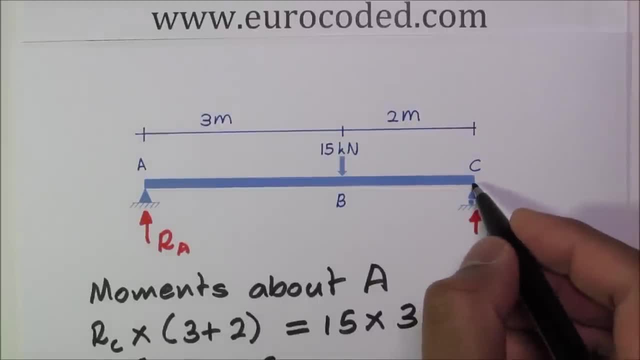 Then we have an anticlockwise moment. It would try to rotate this beam in this direction So we can write moments about C. Then we can take moments about C, Just like before. the lever arm is zero for reaction RC when you are taking moments about C, Hence RC has zero moment about C. Then we have